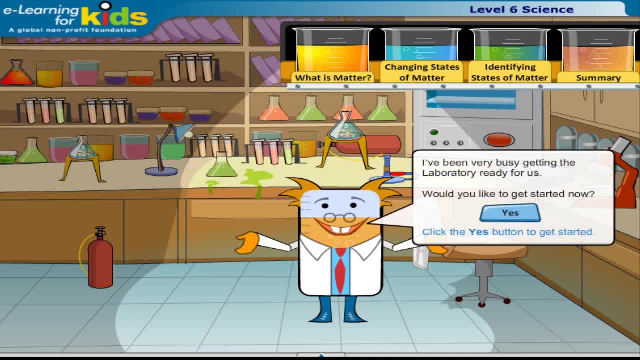 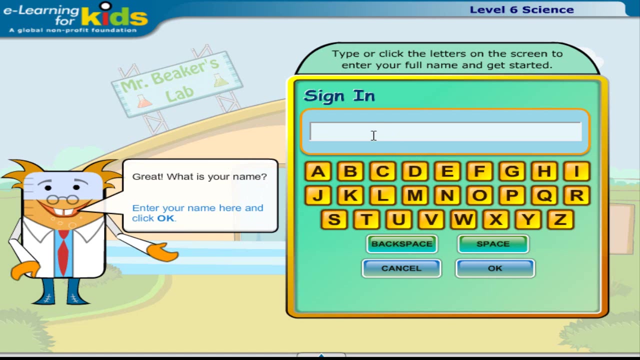 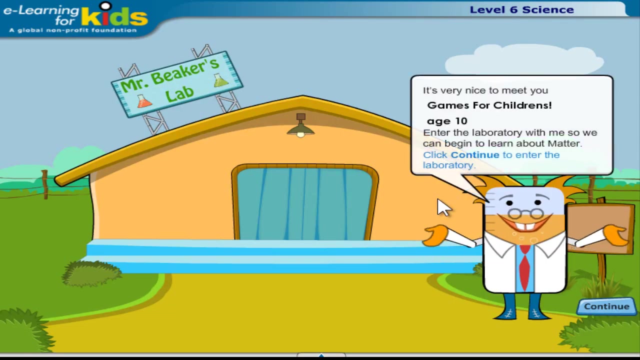 to learn about matter today. I've been very busy getting the laboratory ready for us. Would you like to get started now? Click the yes button to get started. Great, What is your name? Enter your name here and click OK. How old are you? Enter your age here and click OK. 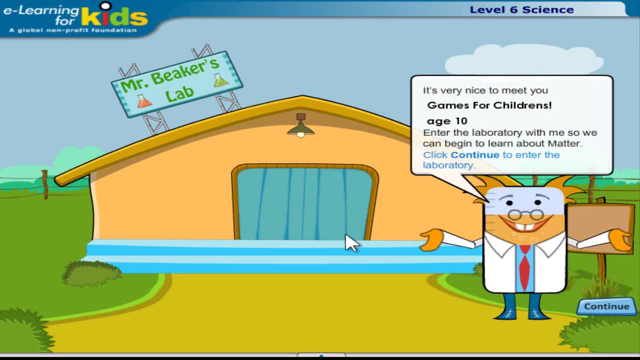 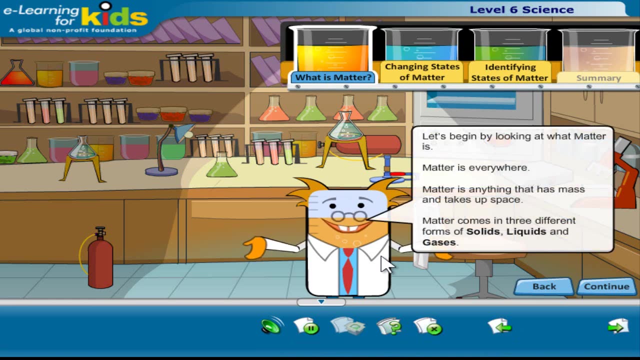 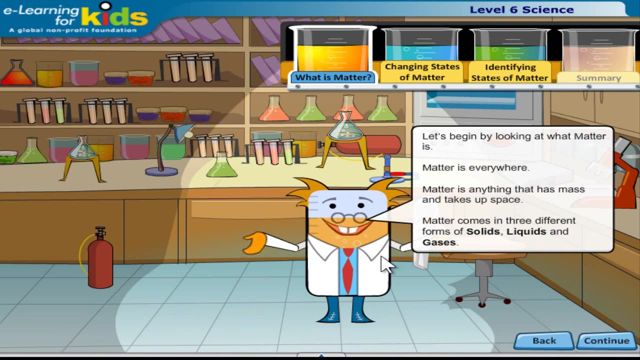 It's very nice to meet you. Enter the laboratory with me so we can begin to learn about matter. Click continue to enter the laboratory. Let's begin by looking at what matter is. Matter is everywhere. Matter is anything that has mass and takes up space. Matter comes in three different forms of solids, liquids. 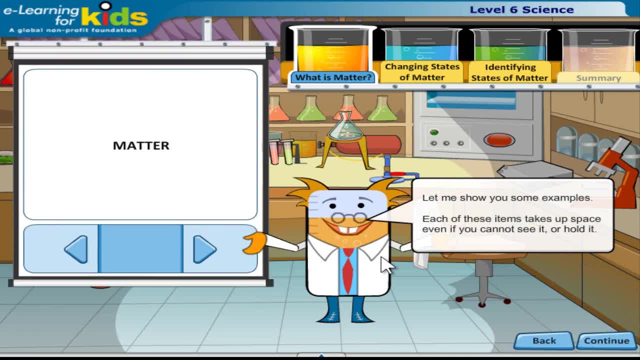 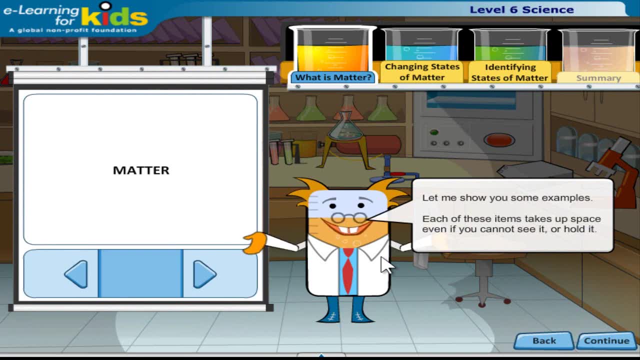 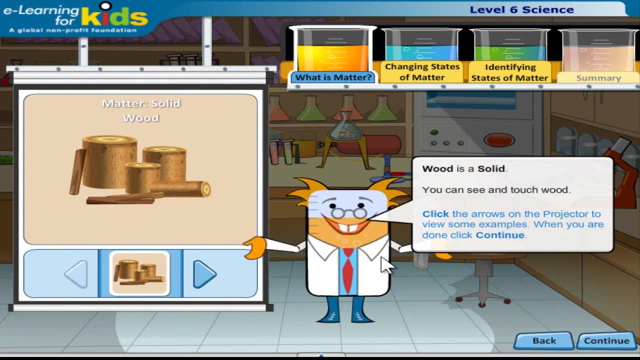 and gases. Let me show you. Let me show you some examples. Each of these items takes up space, even if you cannot see it or hold it. Wood is a solid. You can see and touch wood. Click the arrows on the projector to view some examples. When you are done, click continue. Sand is a solid. Sand is very. 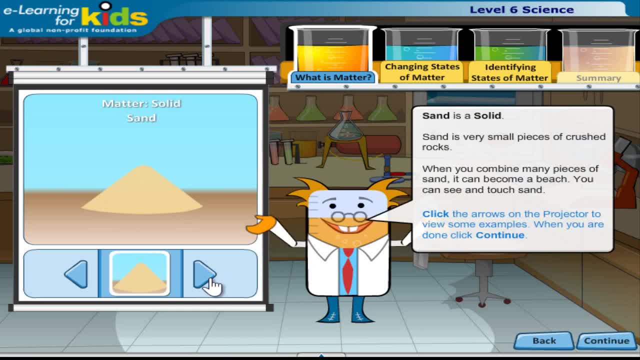 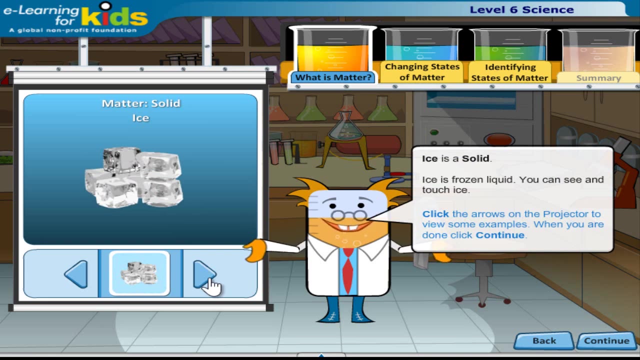 small pieces of crushed rocks. When you combine many pieces of sand, it can become a beach. You can see and touch sand. Click the arrows on the projector to view some examples. When you are done, click Continue. Ice is a solid. Ice is frozen liquid. You can see and touch ice. Click the arrows on. 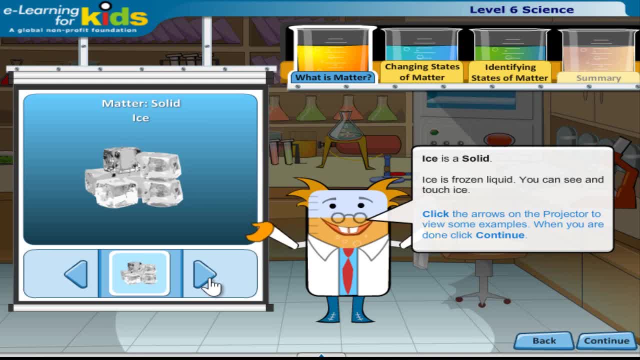 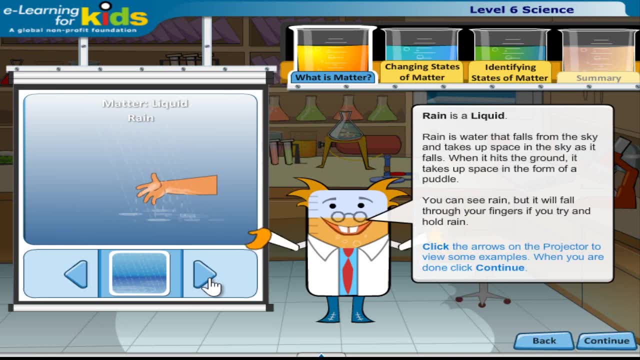 the projector to view some examples. When you are done, click continue, click, continue. rain is a liquid. rain is water that falls from the sky and takes up space in the sky as it falls. when it hits the ground, it takes up space in the form of a puddle. you can see rain, but it will fall through your fingers if you 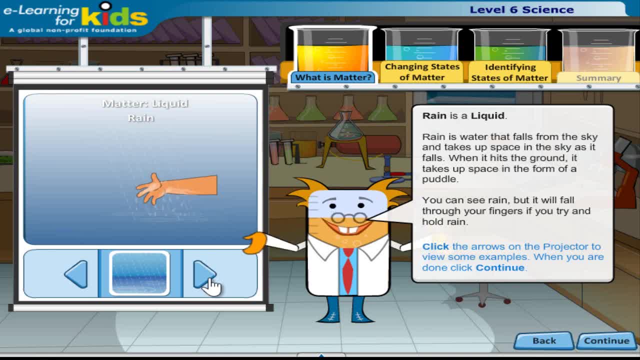 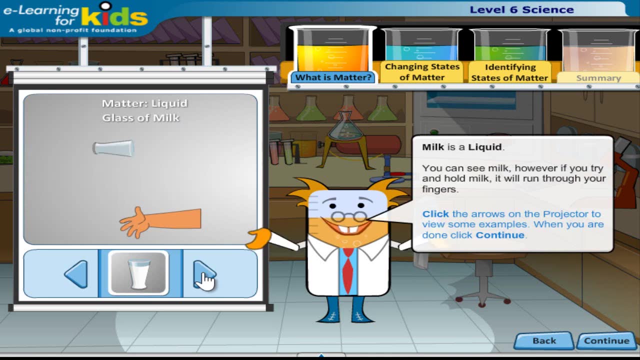 try and hold rain. click the arrows on the projector to view some examples. when you are done, click continue. milk is a liquid. you can see milk. however, if you try and hold milk, it will run through your fingers. click the arrows on the projector to view some examples. when you are done, click continue. 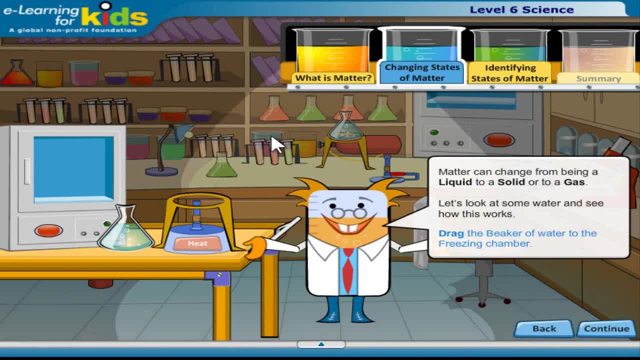 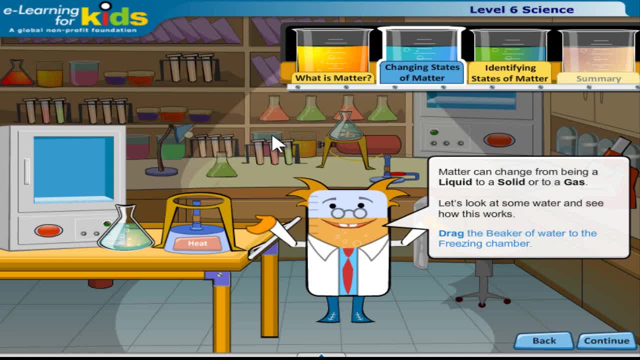 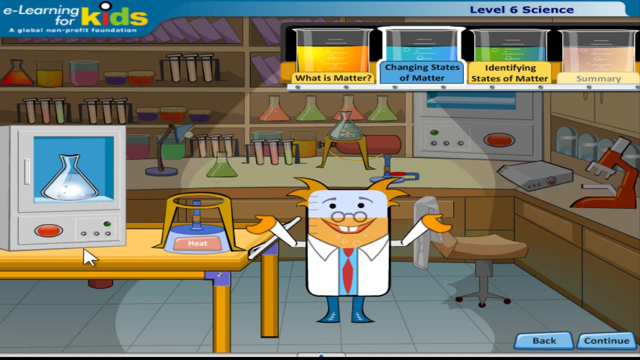 or to a gas. let's look at some water and see how this works. drag the beaker water and see how this works. drag the beaker water and see how this works. drag the beaker of water to the freezing chamber. Good job, Water, when frozen, becomes ice. 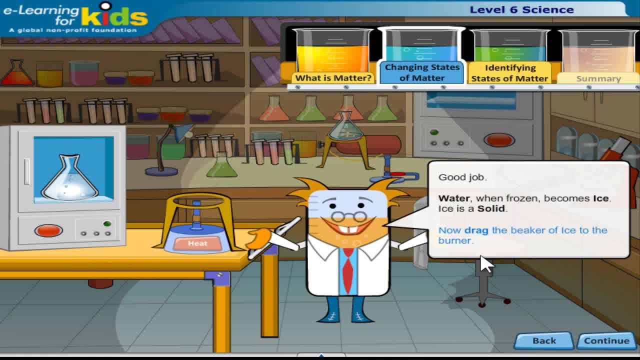 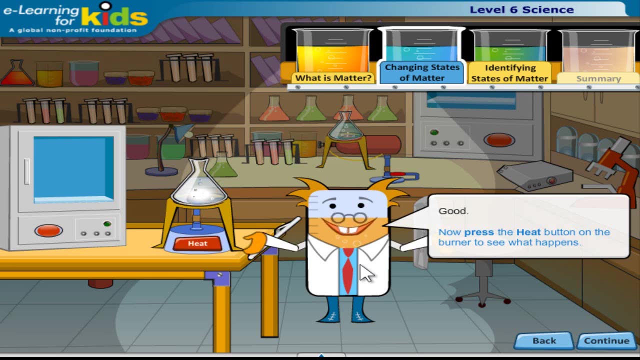 Ice is a solid. Now drag the beaker of ice to the burner. Good, Now press the heat button on the burner to see what happens When the solid frozen water is heated. it becomes liquid again. Press the heat button again to see what happens when we heat the water.